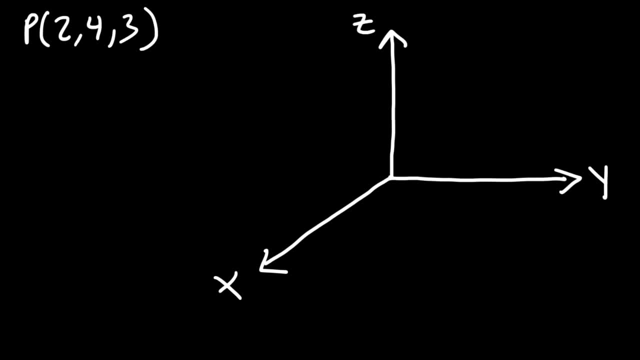 Now to plot the first point, we need to know what is x, what's y and what's z, And it goes in order: alphabetical order: x, y, z. So x is 2.. Let's plot that on the x-axis. 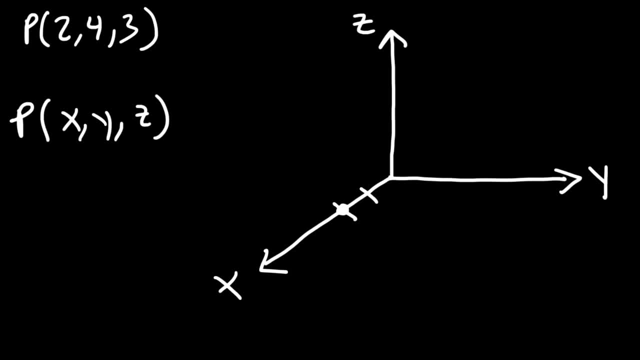 So 2 is somewhere in this region. Now let's plot the y-coordinate, which is 4.. 1,, 2,, 3,, 4.. Here it is. Now. what I'm going to do at this point is draw. 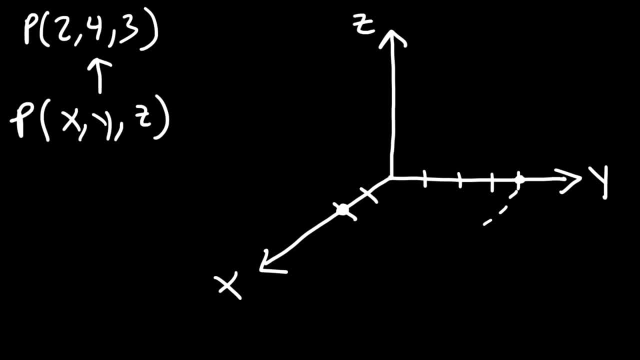 a diagonal. Let's draw a dash line parallel to the x-axis. Let me do this carefully And you can extend it as far as you want. And then, starting with the point, this point here, 2 on the x-axis. 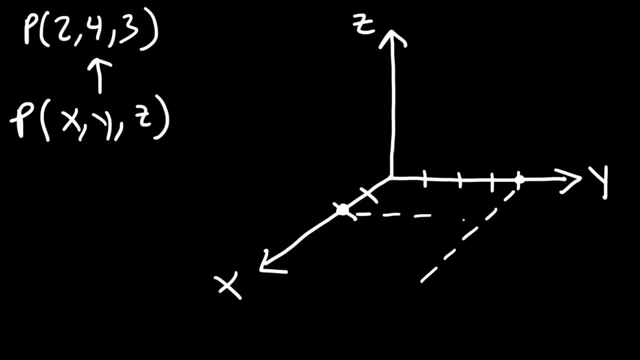 I'm going to draw a dash line parallel to the y-axis, And so where those two dash lines intersect, that's going to be the point of interest. So in the x- y plane I have the point 2, 4.. 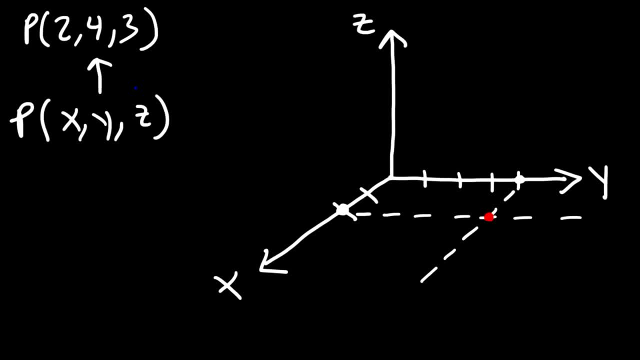 Now the last thing I need is the z coordinate, which is 3.. So let's go up 3 units along the z axis. So I'm going to draw a dashed line that's parallel to the z axis And if you want to, you can just go up 3 units along that dashed line and say that's going to be the point 2,, 4,, 3.. 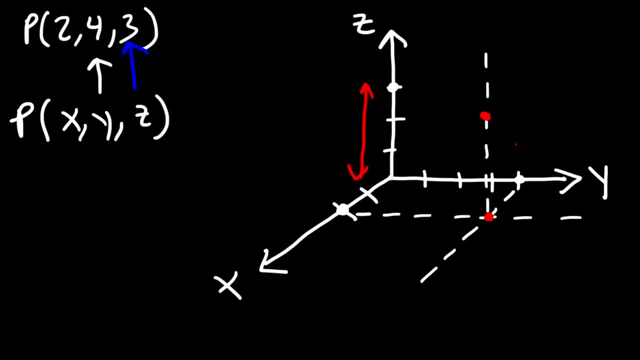 Now you have to make sure that this length is the same as this length here. But if you want to avoid mistakes, here's something else that you could do. Let's take away that point. So what I'm going to do is Travel 2 units along the x axis. 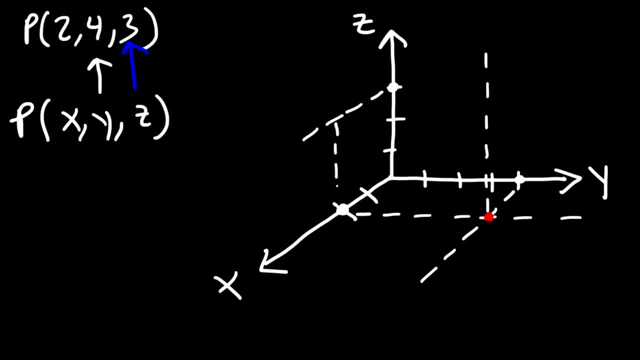 And if you want to, you can draw another line parallel to the z axis here. So this is the next point of interest, And then from that point travel 4 units parallel to the y axis, And so you get this point of intersection. 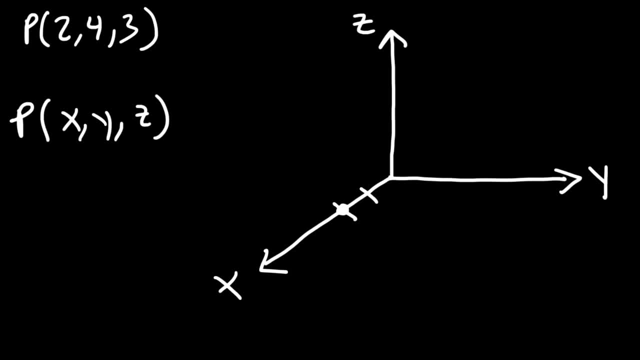 So 2 is somewhere in this region. Now let's plot the y-coordinate, which is 4.. 1,, 2,, 3,, 4.. Here it is. Now. what I'm going to do at this point is draw. 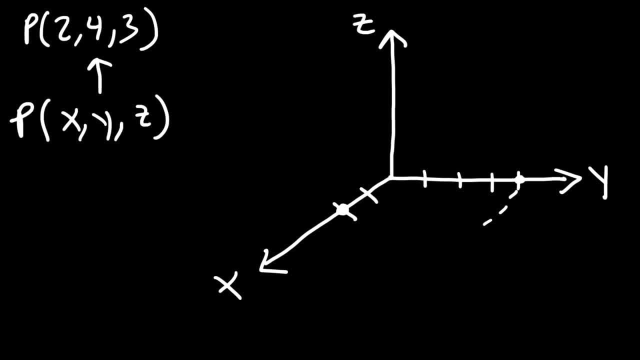 a diagonal. This is a dashed line parallel to the x-axis. Let me do this carefully And you can extend it as far as you want. And then, starting with the point, this point here at 2, on the x-axis, I'm going to draw a dashed line parallel to the y-axis. 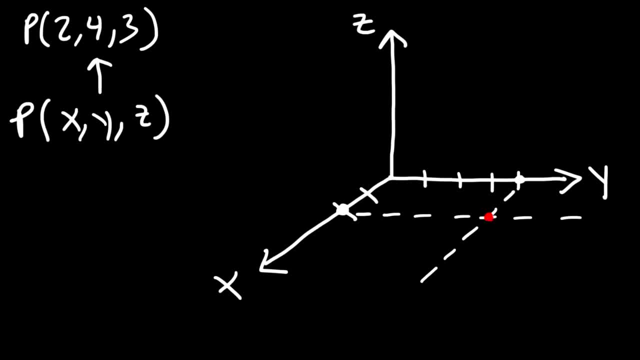 And so where those two dashed lines intersect, that's going to be the point of interest. So in the x- y-plane plane, I have the point. Now the last thing I need is the z-coordinate, which is 3.. So let's go up 3 units along the z-axis. So I'm going to draw a dashed line. 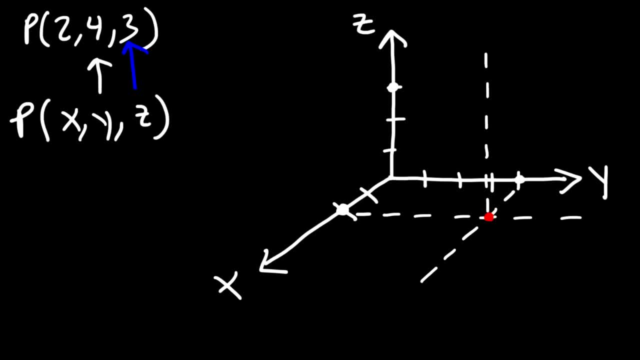 that's parallel to the z-axis, And if you want to, you can just go up 3 units along that dashed line and say that's going to be the point 2,, 4, 3.. Now you have to make sure that this length is the same as this length here. But if you want to avoid mistakes, here's 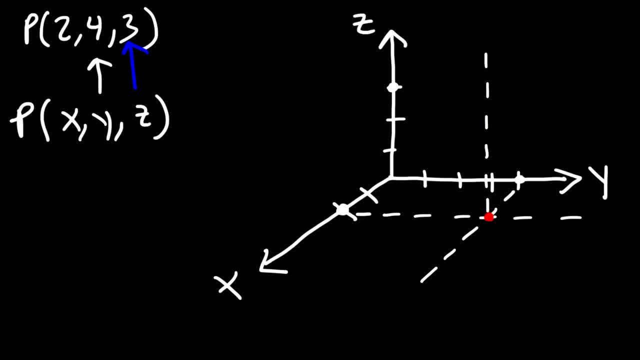 something else that you could do. Let's take away that point. So what I'm going to do is travel 2 units along the x-axis And, if you want to, you can draw another line parallel to the z-axis here. So this is the. 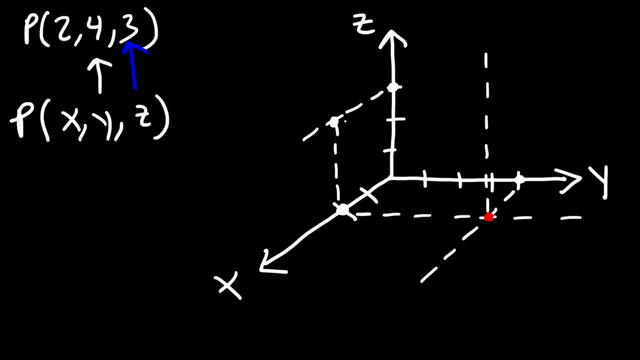 next point of interest And then, from that point, travel 4 units parallel to the y-axis, And so you get this point of intersection, And it is this point that we're looking for. This is point. So, as you can see, we traveled 2 units along the x-axis. 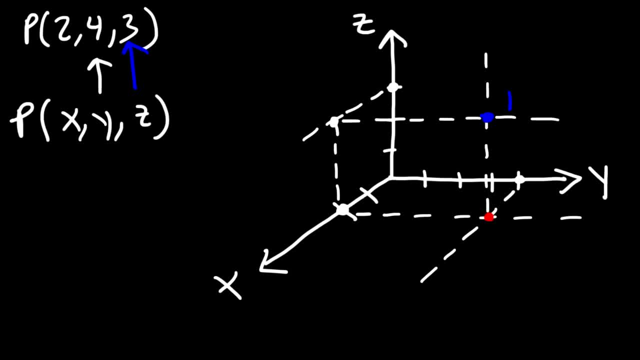 And it is this point that we're looking for. This is point P. So, as you can see, we traveled 2 units along the x axis, And then we traveled 4 units parallel to the y axis And finally, 3 units parallel to the z axis. 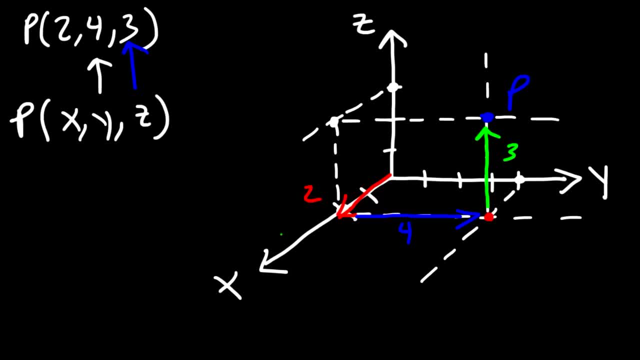 And that will take us to the point 2,, 4,, 3.. And that's basically it. That's how you can graph a point in a 3DX. It's a 3D coordinate system, But for the sake of practice, let's try another example. 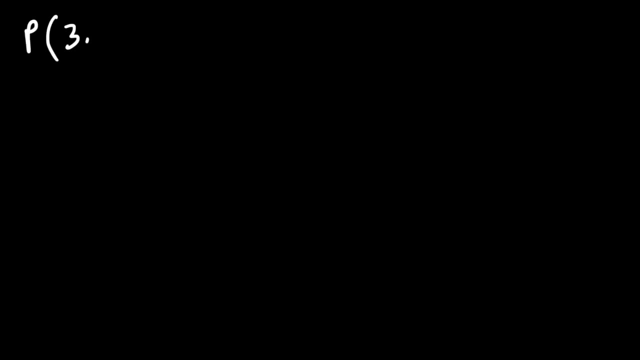 You could try this. if you want, Go ahead and graph the point 3, negative 4, 5.. Feel free to try it. So let's begin by drawing the y axis- Okay, that's not straight- The z axis. 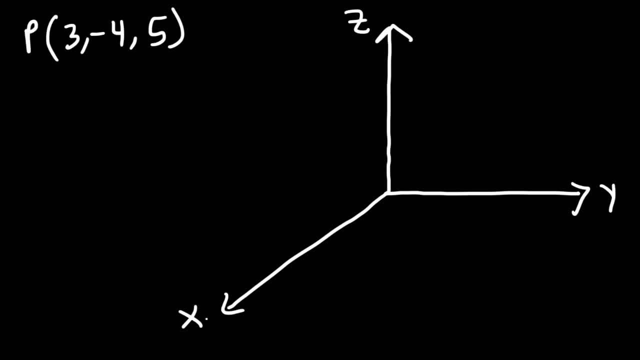 And the x axis. So x is 3,, y is negative 4, and z is 5.. So let's travel 3 units along the x axis. So here it is, And now we need to travel 4 units along the y axis, but we have a negative 4 value. 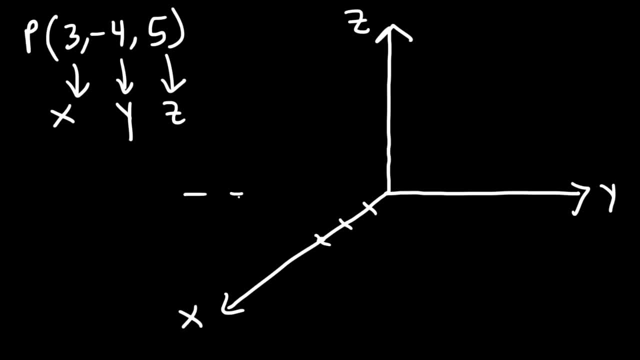 So in this case we need to go in the other direction. If you want to, you could just make it a solid line, So let's travel 4 units this way along the negative y axis. Now we need to find the intersection of these two points. if we draw two parallel dashed lines, 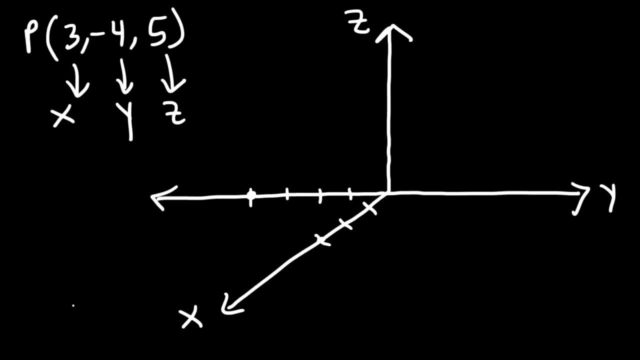 So I'm going to start with this point and draw a dashed line that's parallel to the x axis And then, starting with this point, here we're going to draw a dashed line that's parallel to the x axis. I'm going to draw a dashed line that's parallel to the negative y axis. 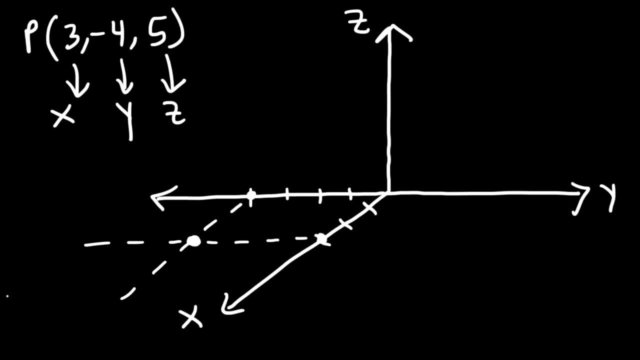 So here is the point of intersection. I'm going to focus on that point. next, Now, let's travel 5 units up along the z axis And, starting with this point here, let's draw a dashed line that's parallel to the z axis. 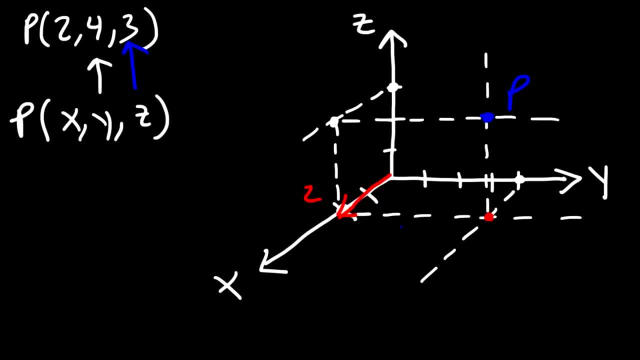 And then we traveled 4 units parallel to the y-axis And finally 3 units parallel to the z-axis, And that will take us to the point, And that's basically it. That's how you can graph a point in a three-dimensional coordinate. 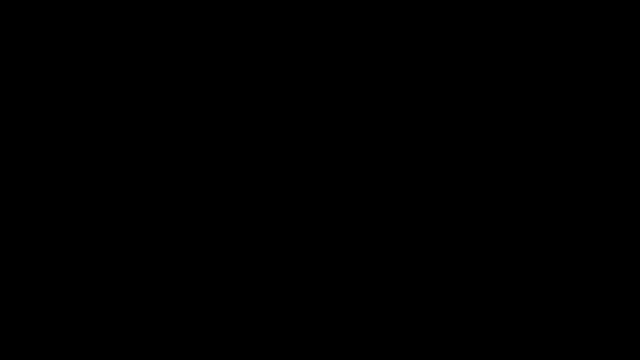 system. But for the sake of practice, let's try another example. You can try this. if you want, Go ahead and graph the point, Feel free to try it. So let's begin by drawing the y-axis. Okay, that's not straight. 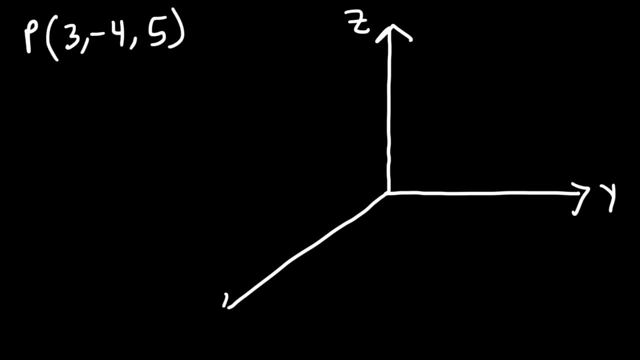 The z-axis And the x-axis. So x is 3.. Y is negative 4. And z is 5.. So let's travel 3 units along the x-axis. So here it is, And now we need to travel 4 units along the y-axis, but we have a negative 4 value. 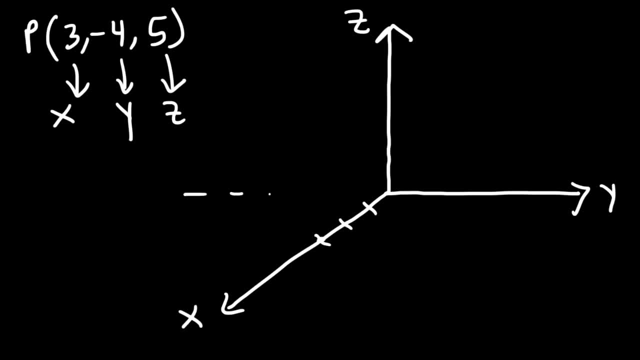 So in this case we need to go in the other direction. If you want to, you could just make it a solid line. Okay, Let's travel 4 units this way along the negative y-axis. Now we need to find the intersection of these two points. if we draw two parallel dash lines, 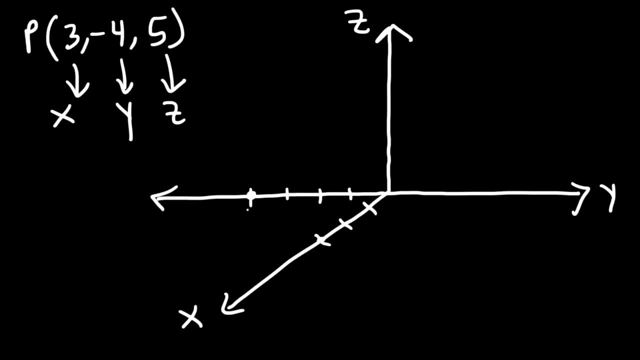 So I'm going to start with this point and draw a dash line that's parallel to the x-axis And then, starting with this point here, I'm going to draw a dash line that's parallel to the negative y-axis. So here is the point of intersection. 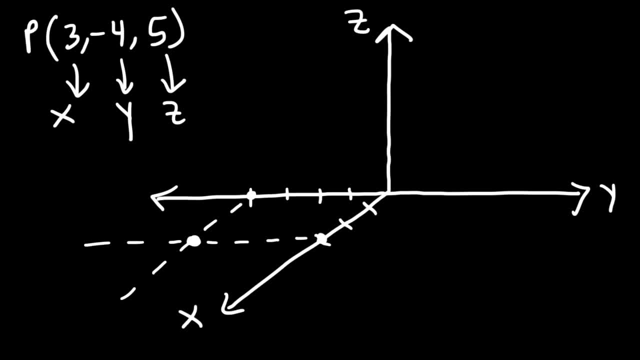 I'm going to focus on that point next. Now let's travel 5 units up along the z-axis And, starting with this point here, let's draw a dash line that's parallel to the z-axis. I know my graph is not perfect.